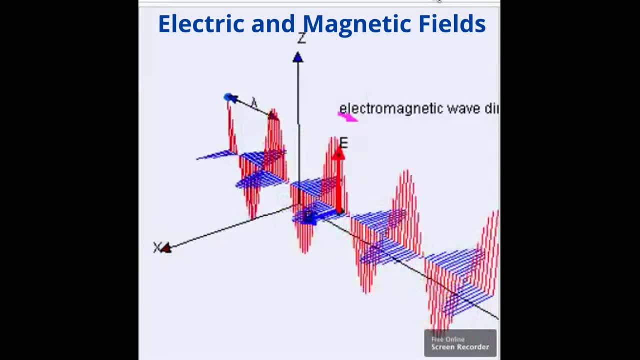 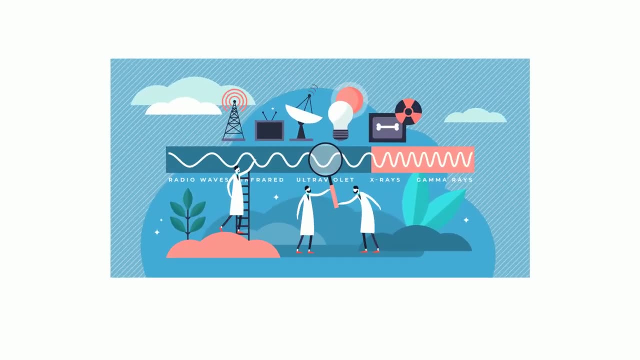 This is why they are called electromagnetic waves. The electric field and the magnetic field of an electromagnetic wave are perpendicular or right angles to each other, and they are also perpendicular to the direction or propagation of the wave. The electromagnetic spectrum is ordered by frequency, which is the number of wavelengths. 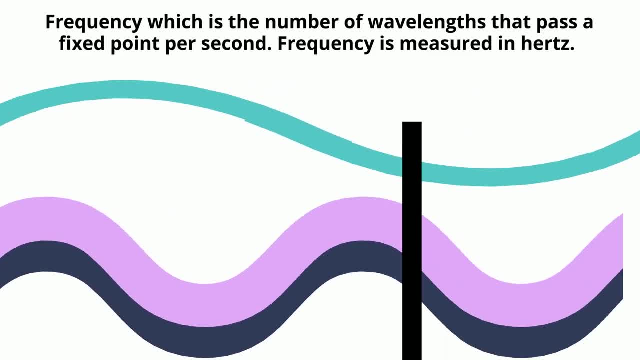 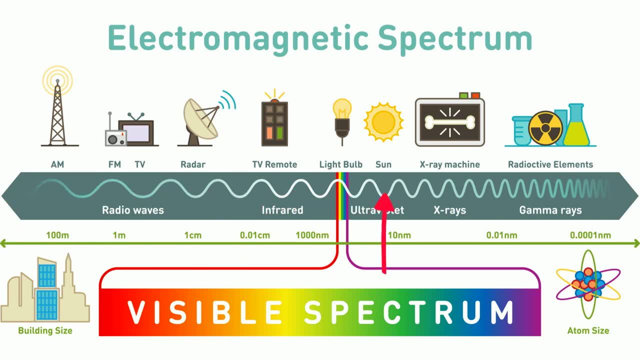 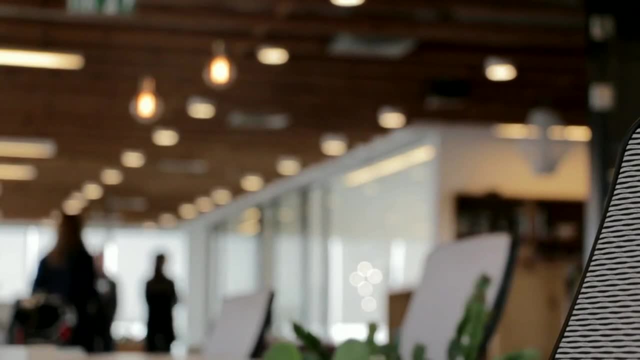 that pass a fixed point per second. Frequency is measured in Hertz. The spectrum has a very wide range from 300 kHz to an incredibly small 3 x 10 to the 21st power Hertz. An electromagnetic wave, can travel through anything like air, solid material or even. 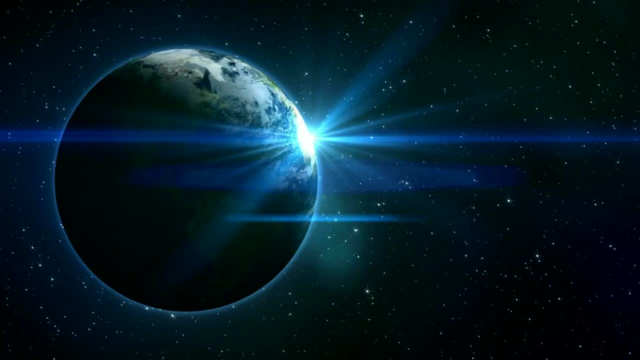 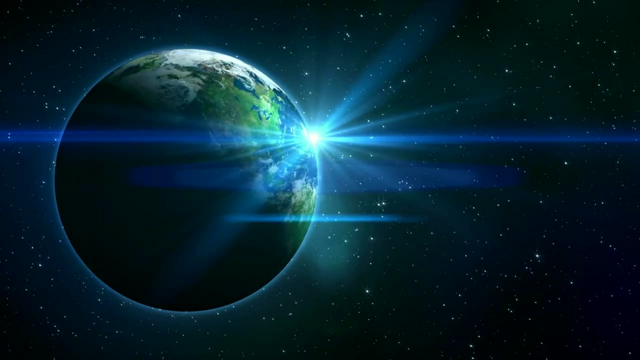 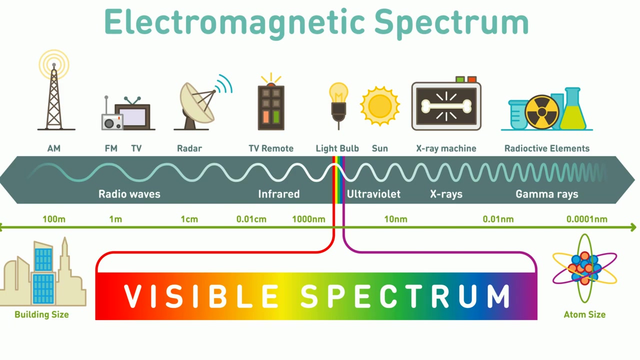 vacuum. It does not need a medium to propagate or travel from one place to another. Electromagnetic waves can even travel through the vacuum of outer space. Let's take a look at the electromagnetic spectrum. Radio waves have a very low frequency and they have a wavelength roughly the size of 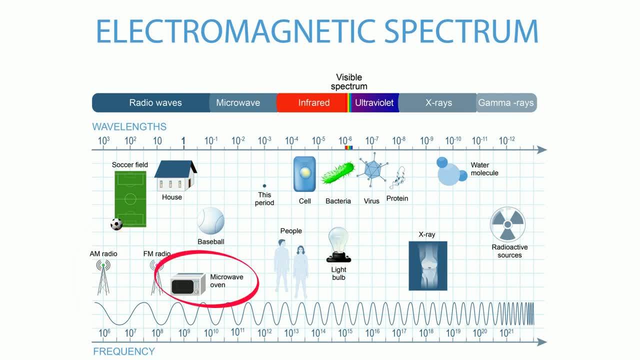 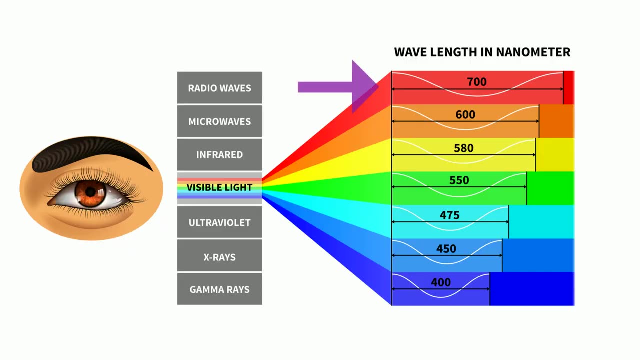 a soccer field. Moving to the right are microwaves and they have wavelengths roughly the size of a baseball. In the middle is visible light, with a wavelength the size of bacteria. Visible light can be subdivided by color, with red having the lowest frequency and blue 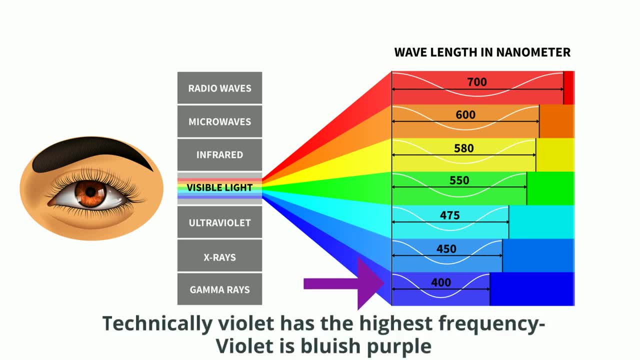 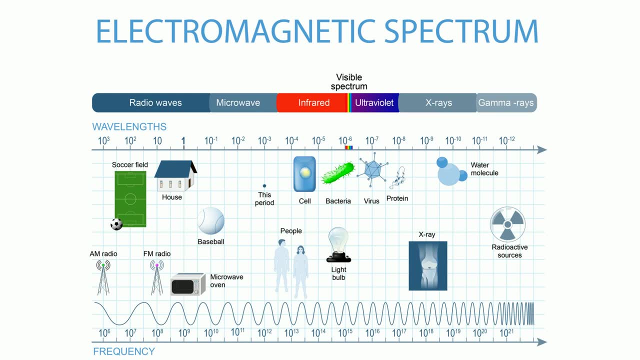 having the highest frequency. The wavelength of the light is very similar to the wavelength of a water molecule. Now, at this point, the wavelengths are very small. X-rays are slightly larger than a water molecule and radioactive sources such as gamma rays are the size of atoms. 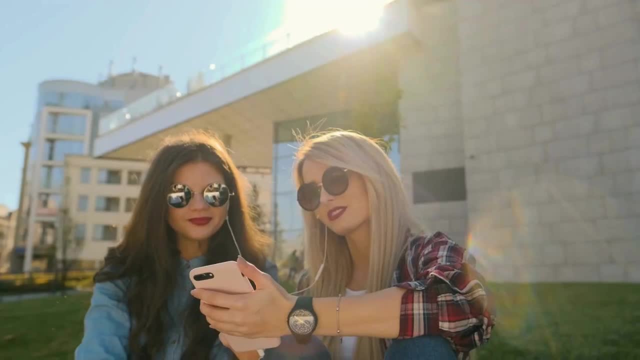 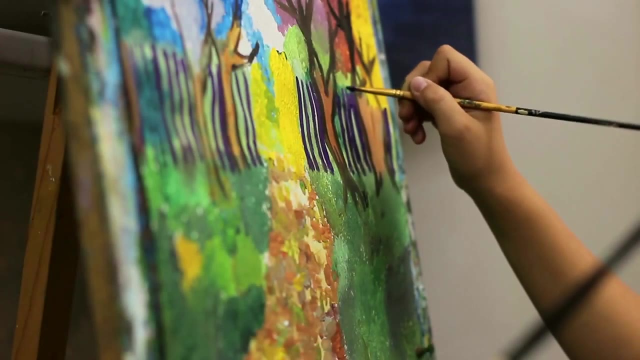 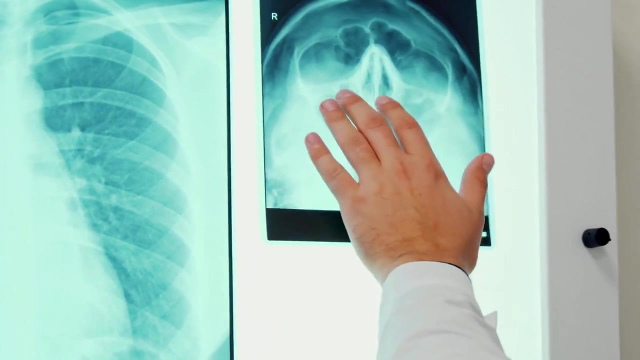 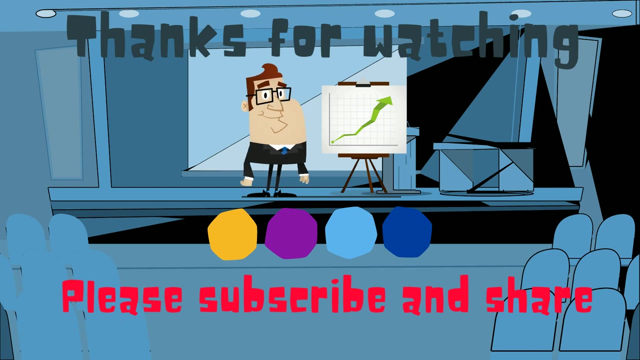 The electromagnetic spectrum is used in every day life, from listening to music, to visible light, to microwave ovens, to even looking inside our bodies. If you would like to know more about the electromagnetic spectrum, this playlist will help. and, as always, thanks for watching. and MooMooMath uploads a new math and science video everyday. Please subscribe and share.